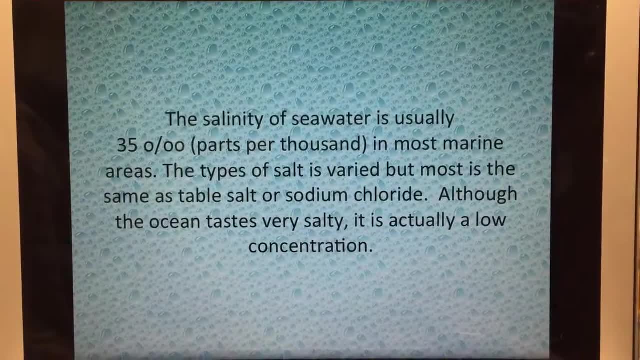 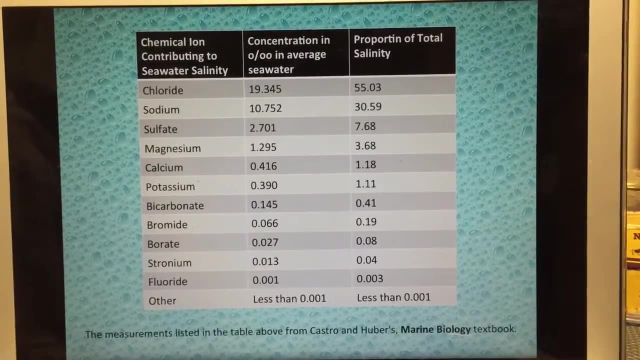 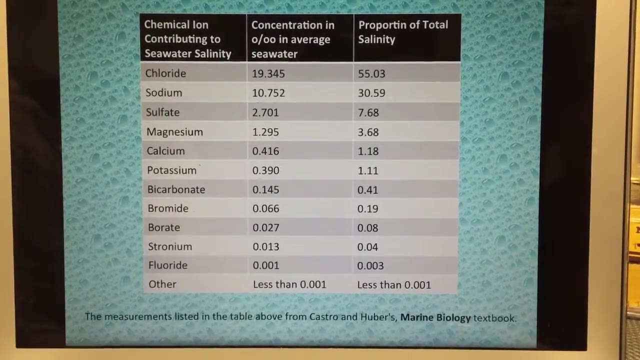 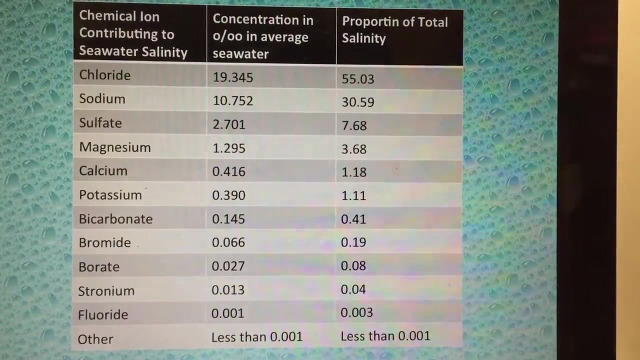 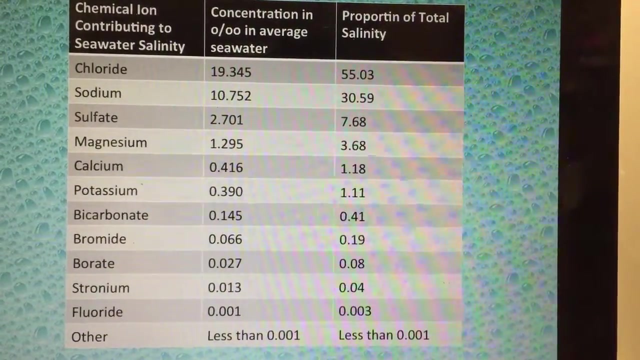 Although the sea tastes very salty, it is a low concentration. The brightness of the colors clearly бум conveys seawater salinity card outfits. they are not directly salt. Chemical ions include chloride at 19.345 parts per thousand and the proportion of salinity is 55.. The chemical ion proportion of 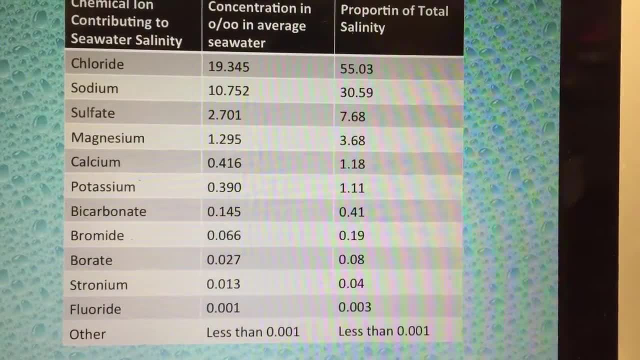 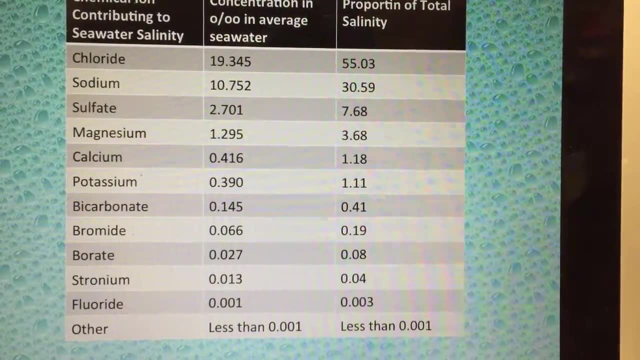 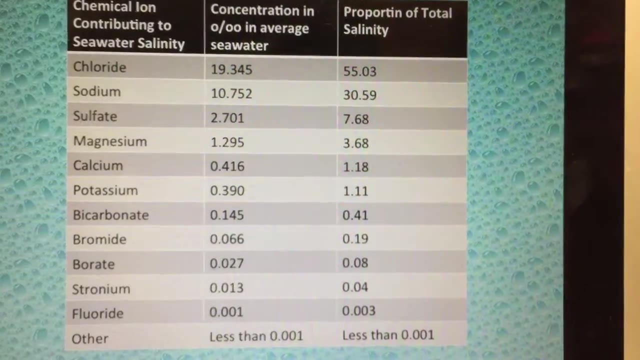 salinity then goes down from here, From chloride to sodium, sulfate, magnesium, calcium, potassium, bicarbonate, bromide, borate, strontium, fluoride and other chemical ions. The lowest amount of concentration in the average seawater is for other. 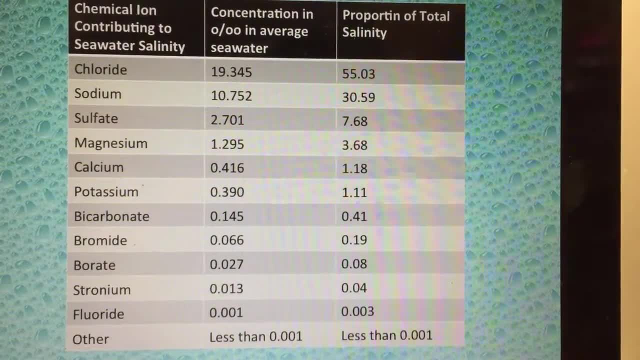 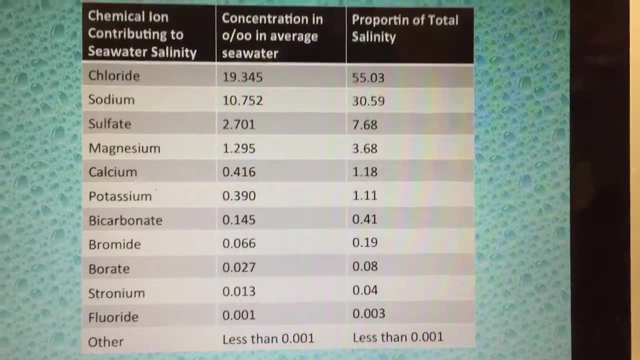 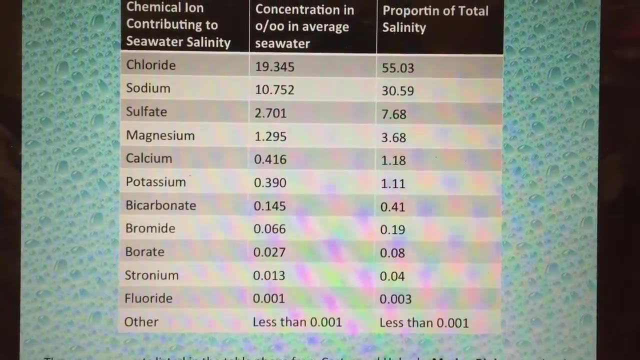 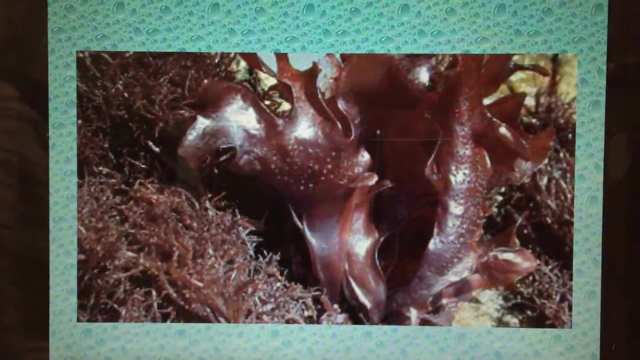 chemical ions at less than 0.001 parts per thousand, with a proportion of total salinity at less than 0.001 parts per thousand. The measure Instruments listed in the table above come from Castron Huber's Marine Biology textbook. Variations occur in ocean salinity due to several factors. The most common factor is the relative amount of evaporation or precipitation in an area. If there is more evaporation than precipitation, the salinity increases. If there is more precipitation than evaporation, the salinity decreases. Another factor that can change the salinity in the ocean is due to a very large river. 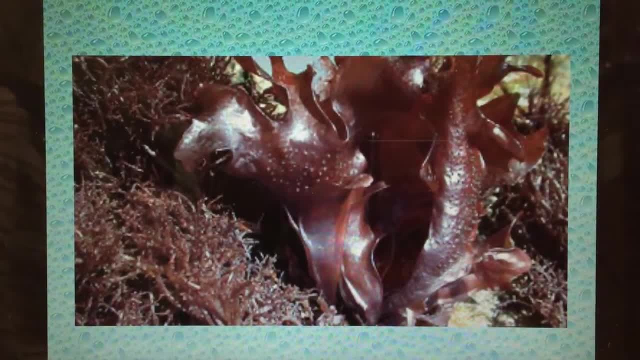 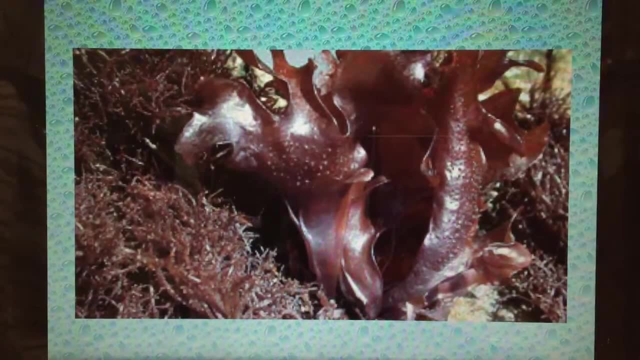 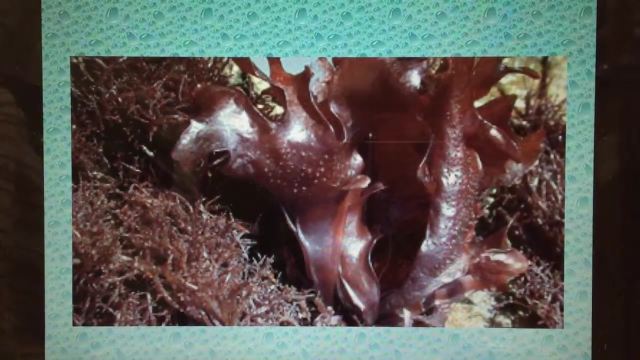 emptying into the ocean. The runoff from most small streams and rivers is quickly mixed with ocean water by the currents and has little effect on salinity. But larger rivers like the Amazon River in South America may make the ocean have little or no salt content for over a mile or more out to sea. 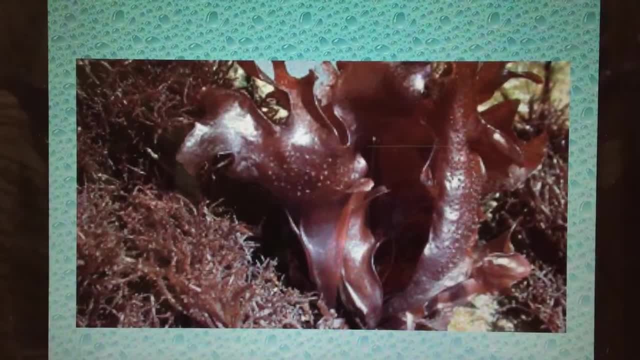 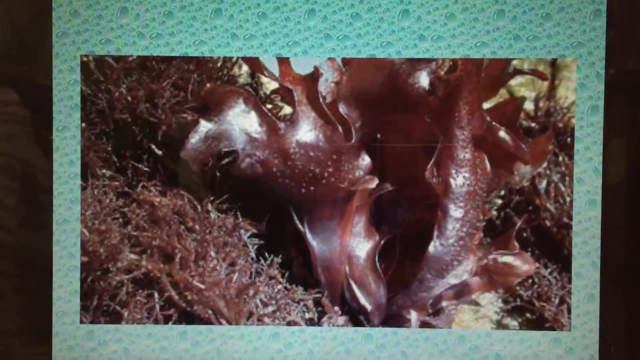 The freezing and thawing of ice also affects salinity. The thawing of large icebergs may affect salinity Instead of frozen. fresh water and lacking any salt, will decrease the salinity, while the actual freezing of salt water will increase the salinity temporarily. 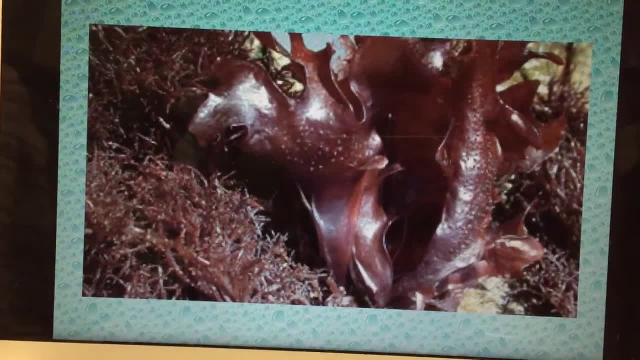 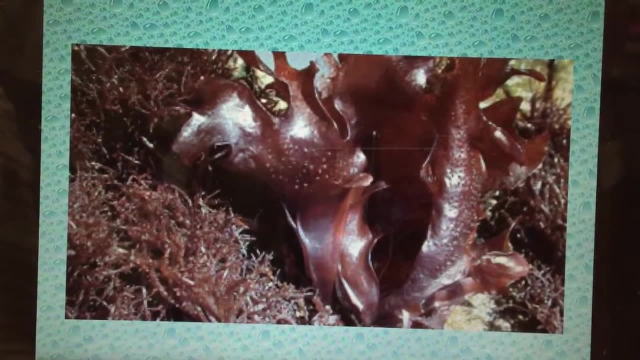 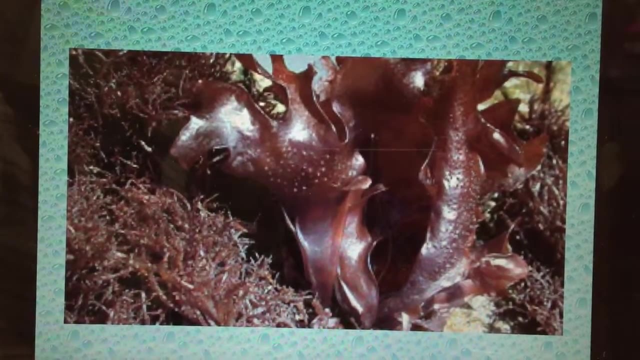 This temporary increase happens in the first stages of the freezing of seawater, when small ice crystals form at about minus two degrees centigrade. These tiny, needle-like ice crystals are frozen fresh water and the salts are not part of them, so the liquid between these crystals becomes increasingly salty, to the point of 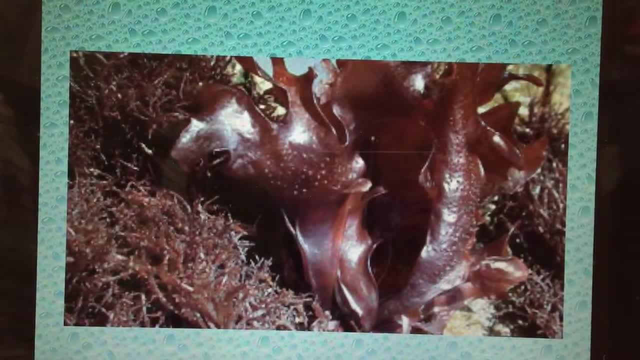 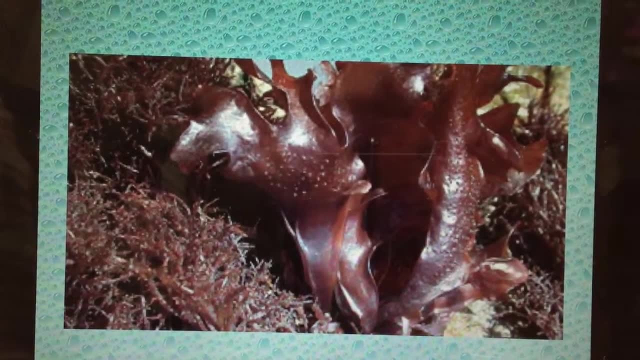 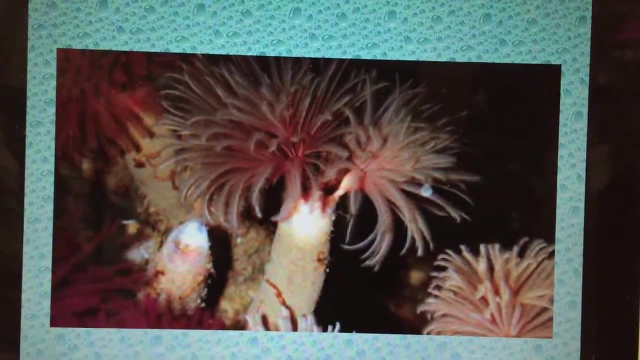 it being in the ocean. Eventually, though, as seawater freezes the ice crystals, tap areas with brine and the entire large piece of frozen seawater, ice flow is salty. Many marine organisms are highly affected by changes in salinity. This is because of a process called osmosis, which is the ability of water to move in and 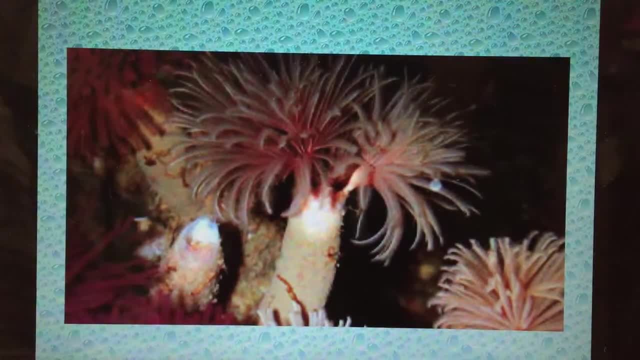 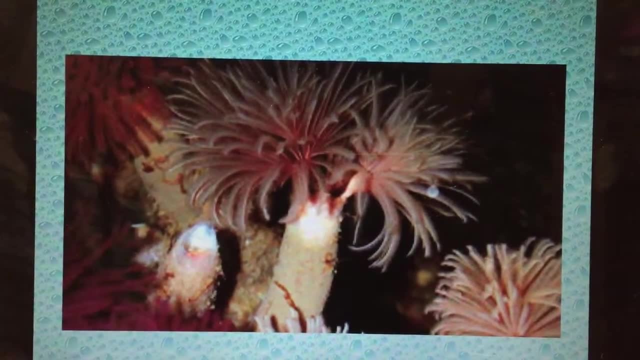 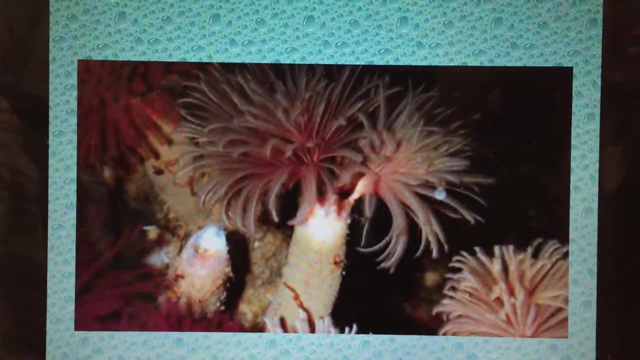 out of living cells in response to a concentration of a dissolved material until an equilibrium is reached. In general, the dissolved material does not easily cross the cell membrane, so the water flows by osmosis to form an equilibrium. Marine organisms respond to this as either being osmotic conformers, also called poikilosmotic. or osmotic regulators or homeoosmotic. The temperature of seawater varies with the amount of sun that hits that area. The temperature of seawater varies with the amount of sun that hits that area. The temperature of seawater varies with the amount of sun that hits that area. 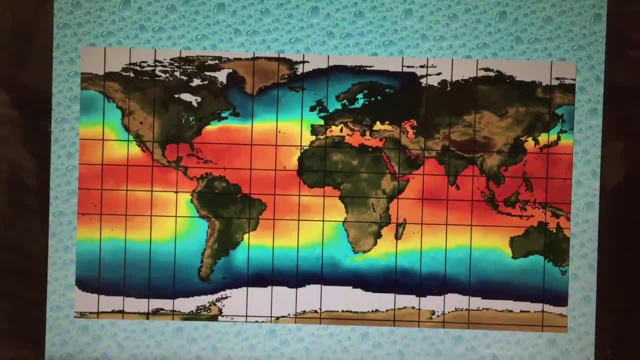 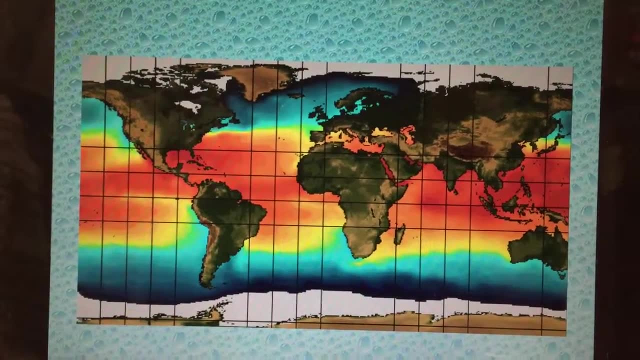 This includes the length of time as well as the angle of the sun's rays. The longer the time and the more direct the rays of sun fall in the ocean, the greater the temperature of seawater. Thus, tropical areas that get more year-round sun and more direct sun, around 90 degrees. 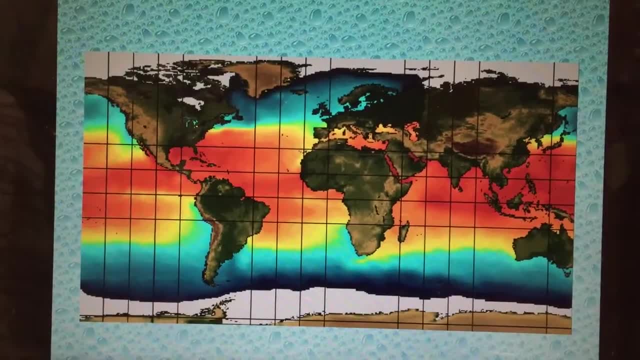 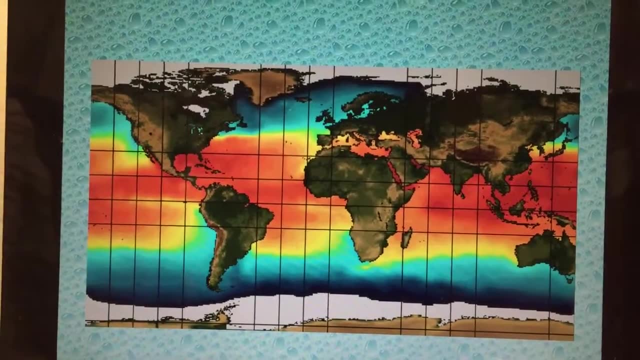 straight down for most of the year at noon, have warmer surface water than polar areas that may have no sun at all for several months each year, and the very steep angles of the sun's rays. Knowing this about ocean water, I would like to say that the temperature of seawater is 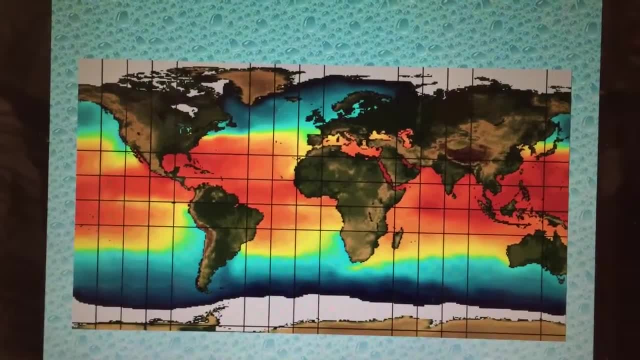 about 30 degrees to about 20 degrees to theaton. Knowing this about ocean water, I would like to say that the temperature of seawater is about 30 degrees to about 20 degrees to theaton. Knowing this about ocean water helps us understand that surface ocean temperatures are warm in. 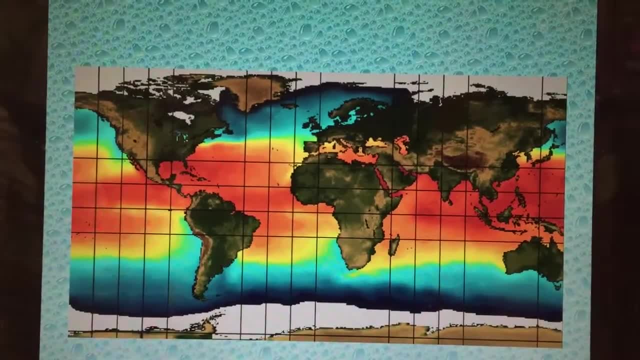 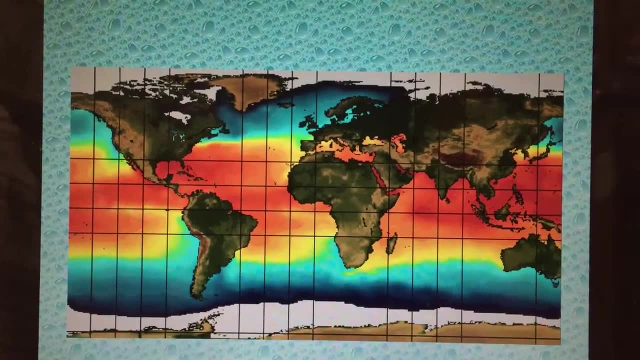 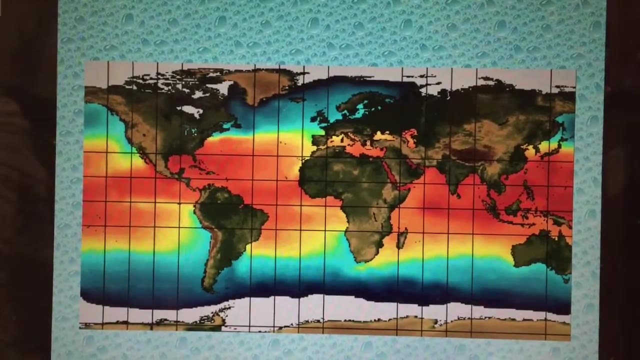 the tropics and cooler at the poles, down to 2.6 degrees. but when we look below the surface we find that the oceans are also vertically stratified and marine scientists recognize a basic three-layered ocean: the upper mixed layer, the main thermocline. 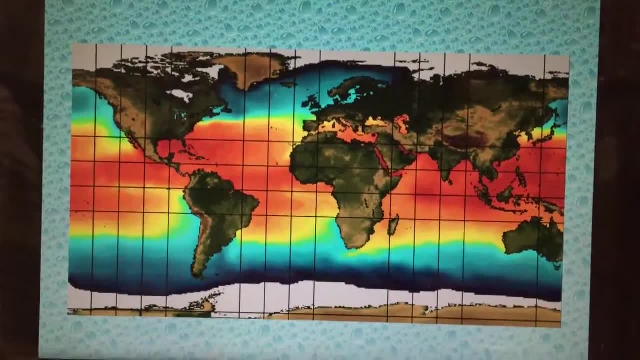 and the deep bottom layer. The sea water temperature affects marine organisms by changing their날, by changing their natural parameters. Knowing this about ocean water helps us understand that surface ocean temperatures are warm in the tropics 70 or more degrees Celsius, and cooler at the poles, down to negative. 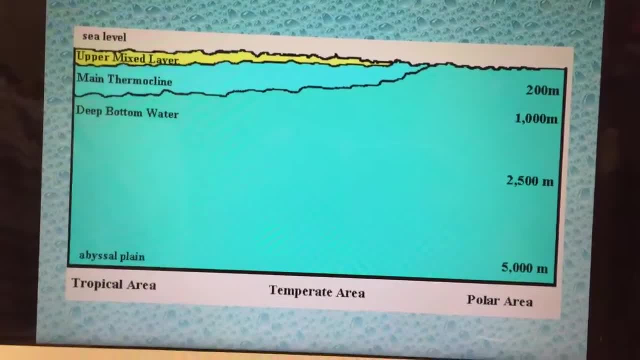 mechanisms by changing the reaction rates within their cells, although each specific